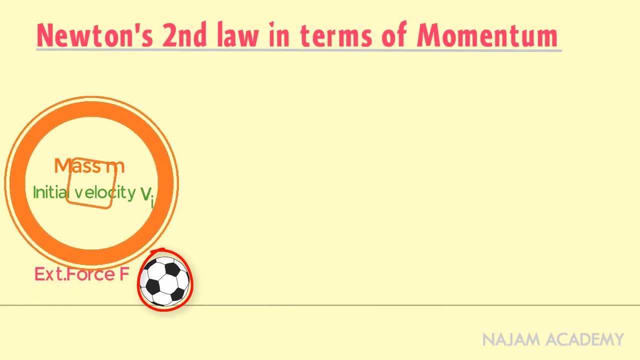 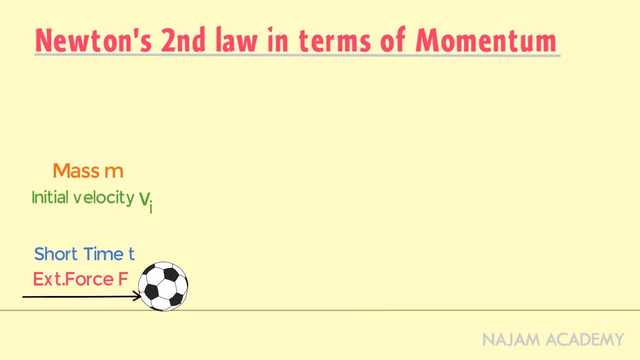 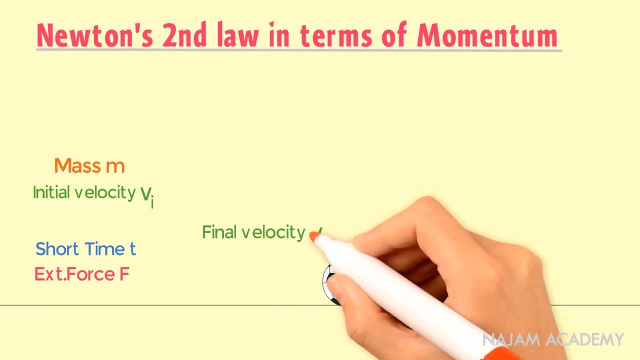 an external force. F acts upon it for a short time. p and this direction. Due to this applied force, the initial velocity of an object would be changed. As a result, the ball will start moving with final velocity vf. Or you can say this trick Whenever the object of mass 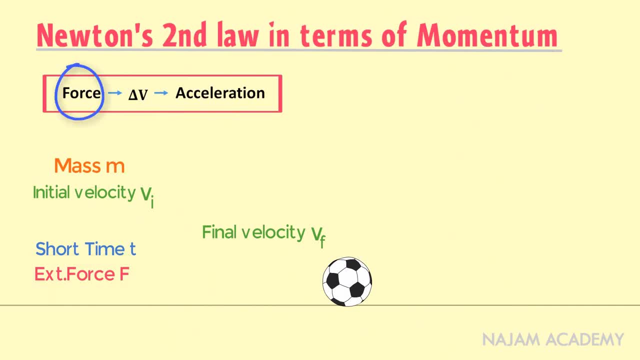 m is moving with initial velocity of vi. the initial velocity of the object is changed. In this way, the velocity of the object is moved. However, if you exert some sort of force on an object, its velocity will be changed. Our velocity changes due to applied force. 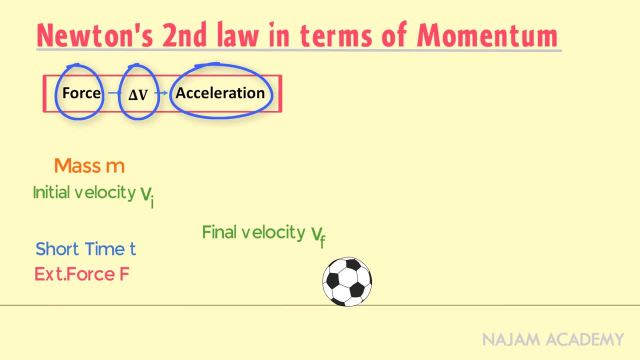 When velocity changes, acceleration produces in a body. Thus, according to Newton's second law, F is equal to m, a or a is equal to F divided by m. Now, this is equation number 1.. Now, mass m, acceleration, A is produced. If you ask why, the answer is that this force 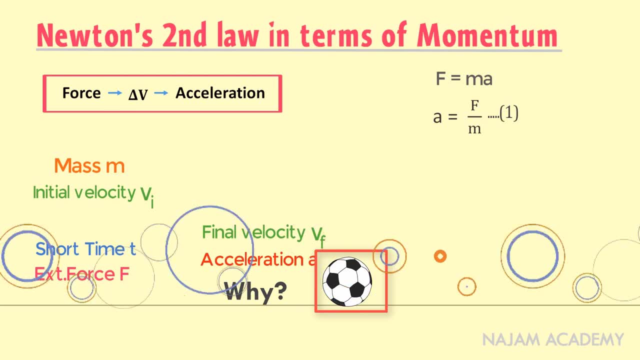 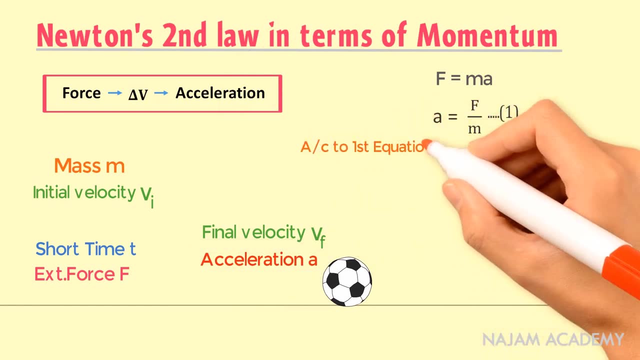 changed the velocity of this object. As a result, or according to this magic trick, acceleration A is produced in this object. According to first equation of motion, acceleration is equal to Vf minus Vi divided by time. Let. this is equation number 2.. Now putting equation number 2 and equation number 1, thus, instead of A, 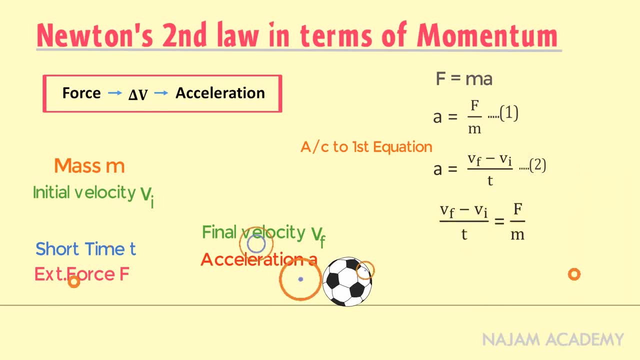 we will write: Vf minus Vi divided by T is equal to F divided by m, or F N to T is equal to MVF minus MVI. This shows that the force acting for short time, T, will cause to change the momentum of this object. 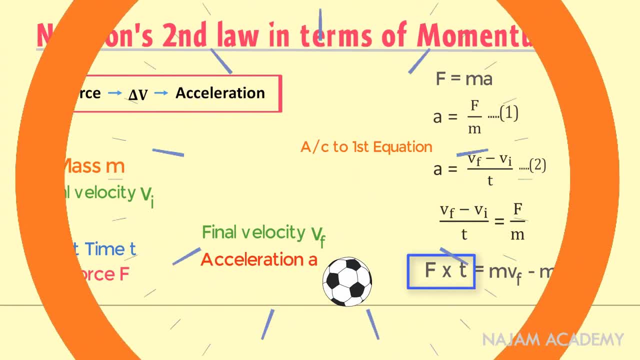 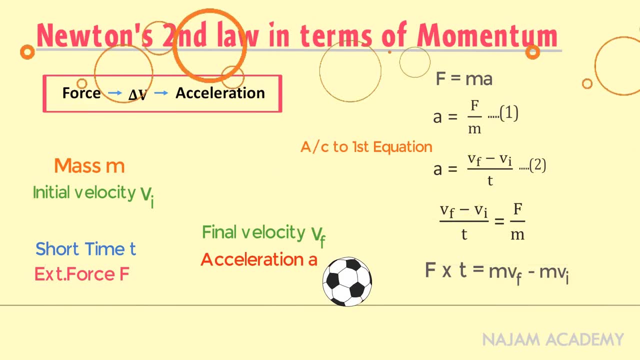 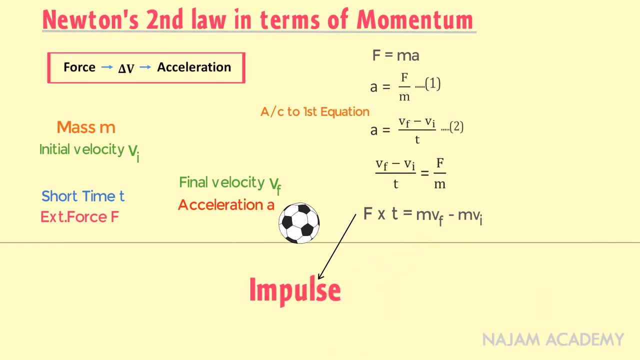 object. it also means that the product of force and time is equal to change in momentum. or we can write: the product of force and time is equal to pf minus pi. remember that the product of force and time is also known as a impulse, which is equal to change in momentum. later in the lecture, 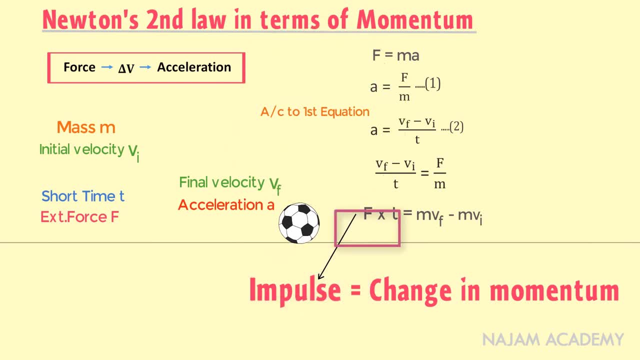 or whenever you listen, impulse. it will be the product of force and time and it will be equal to change in momentum. you can simply say that impulse changes momentum of an object. now let me teach you one final concept required for the derivation of law of conservation of momentum. 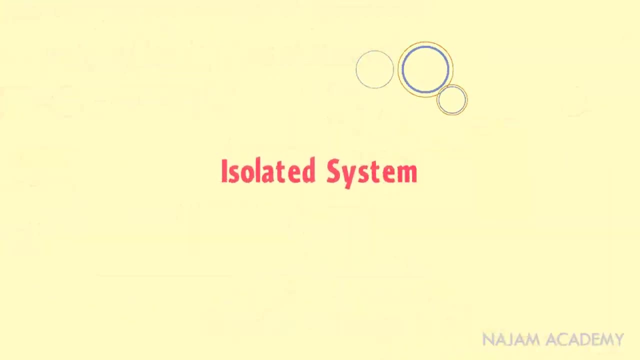 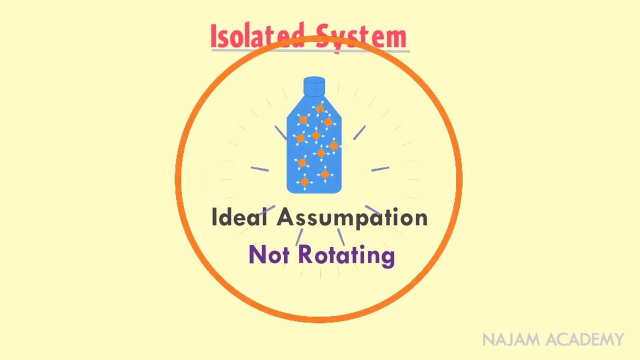 that is isolated system. isolated system. let's consider that a bottle is filled with gas and the piston of the bottle is tightly sealed. now the gas particles or molecules are free to move within the bottle. here we make an ideal assumption that these molecules are not rotating about their axes. they just keep their one directional movement and they do not. 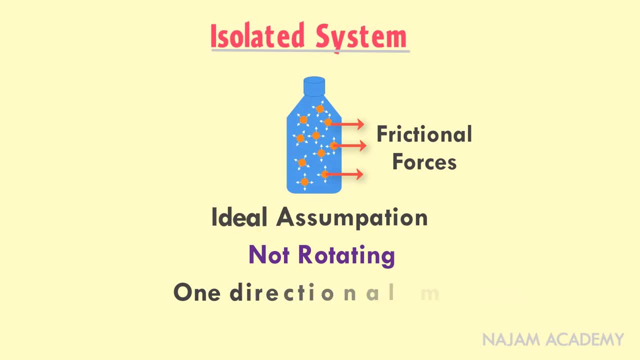 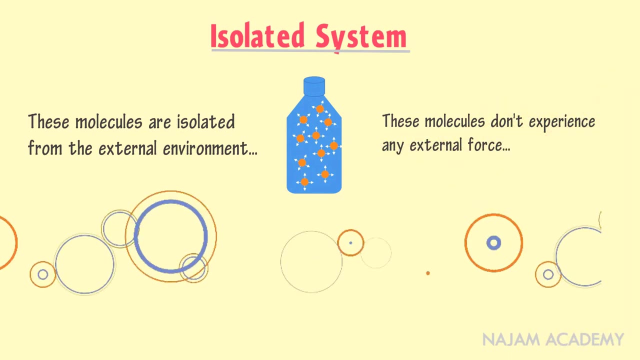 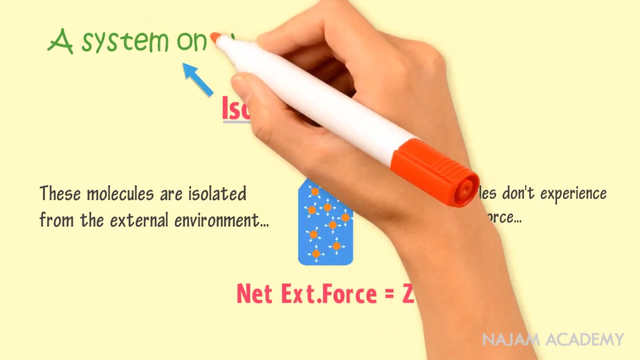 experience any sort of fractional forces during collision. thus these molecules are isolated from the external environment. or we can say that these molecules of gas do not experience any external force, or the net external force on these molecules are zero. thus this system of molecules and physics is known as a isolated system. simply remember that isolated system is a system on which 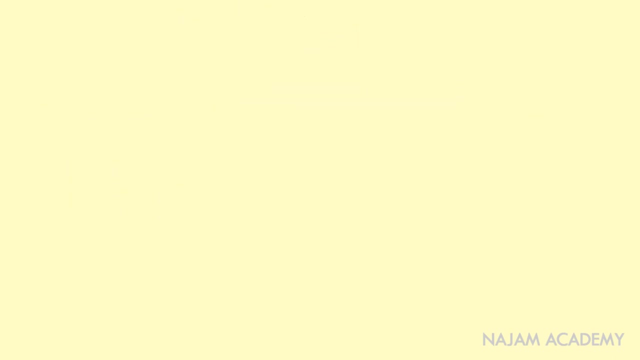 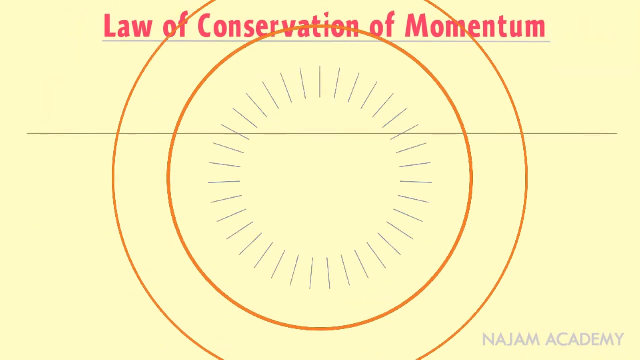 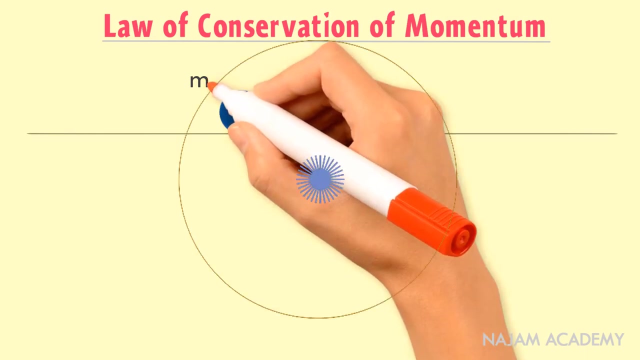 no external force acts. now let me derive the law of conservation of momentum. suppose there is an isolated system in which two balls are moving in this direction. let the mass of this object is m1 and the mass of this object is m2. let the initial velocity of this object is u1. 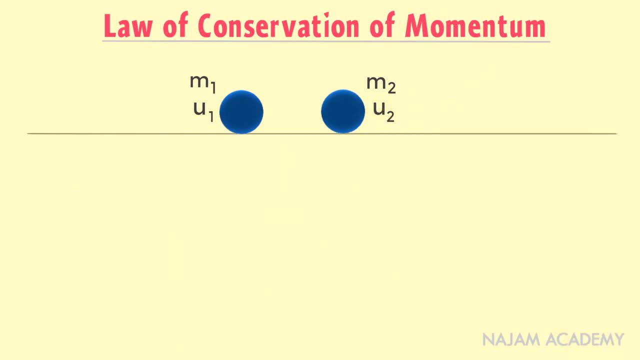 and the initial velocity of this object is u2. let the initial velocity of this object is u2. let the initial velocity of this object u1 is greater than u2. it mean, as these two objects continue their motion, there will be a time when ball m1 will collide with ball m2. if you think why. 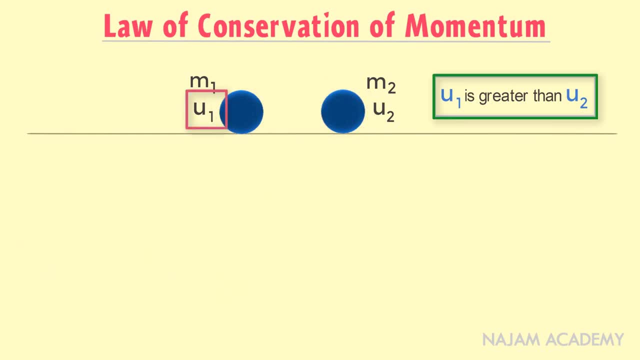 the answer is that initial velocity u1 of ball m1 is greater than initial velocity u2 of ball m2. hence ball m1 is moving faster than ball m2. that's why they will collide at some point during their motion. during collision, the ball m1 will exert force f1 on the ball m2. 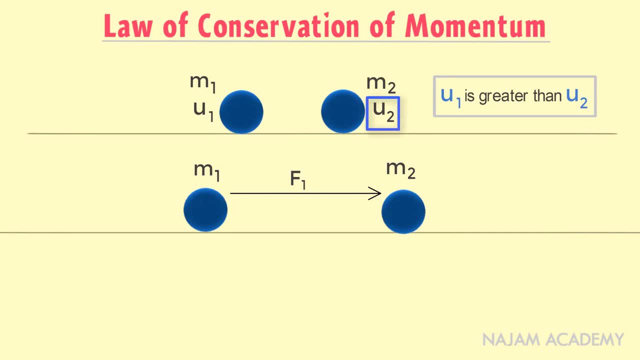 hence the initial velocity u2 of ball m2 will change and to final velocity v2 due to the applied force f1. Now, according to Newton's third law of motion, if ball M1 exerts force on ball M2, then the ball M2 will also exert force F2 on ball M1. 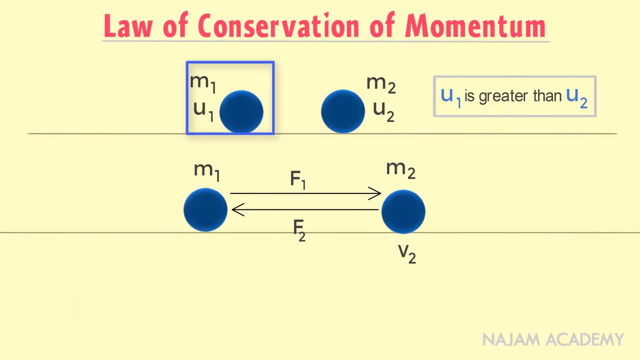 Hence the initial velocity U1 of ball M1 will be changed into final velocity V1. Thus F1 and F2 are action and reaction. Now let me find the respective momentum of these balls. The initial momentum of ball M1 is Pi, is equal to M1 into U1 and the initial momentum of 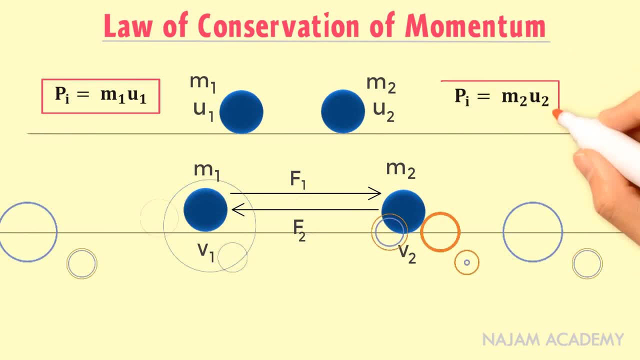 ball. M2 is. Pi is equal to M2 into U2.. During collision the momentum of both the balls changed. Can you guess why I am stating so? I hope you know the answer. It is because during the collision, both the balls experienced impulse. 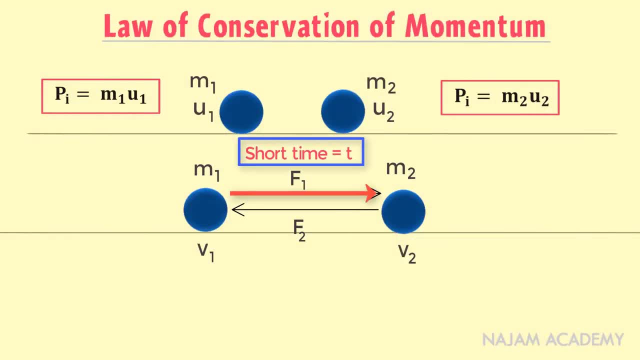 It means F1 acts for short time T on M2 and F2 also acts for short time T on M1.. As a result, the momentum of both the balls changed due to the impulse they experienced. Hence the momentum of M1 is P is equal to M1, V1.. 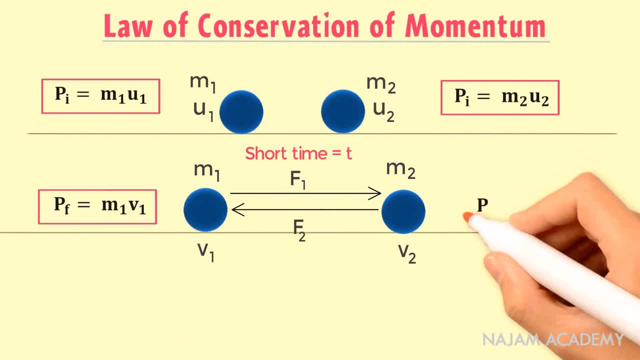 Now let me find the initial momentum of both the balls. The initial momentum of ball M1 is Pi is equal to M2- V1. and the final momentum of ball M2 is P is equal to M2- V2.. Thus the impulse F1 into T changed the momentum of M2.. 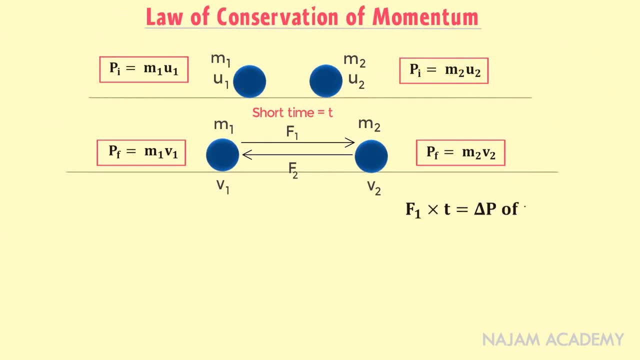 Hence the product of F1 and T is equal to change in momentum. R F1 into T is equal to M2 V2 minus M2 U2.. This is equation number 1.. While the impulse F2N2T change the momentum of M1, thus F2N2T is equal to change in momentum. 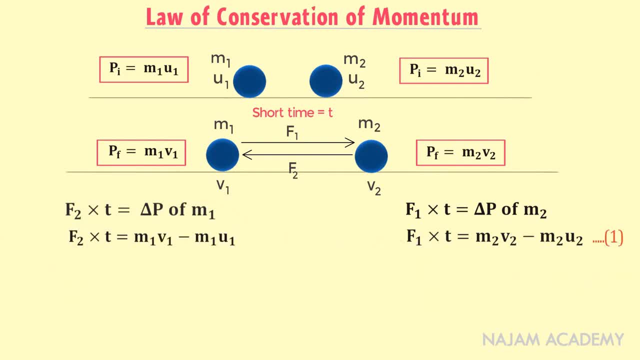 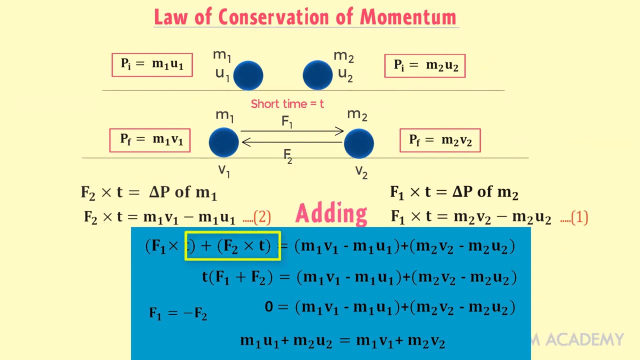 or F2N2T is equal to M1 V1 minus M1 U1.. Let, this is equation number 2.. Now adding equation number 1 and equation number 2.. F1- N2T plus F2 N2T is equal to M1 V1 minus M1 U1 plus M2 V2 minus M2 U2.. 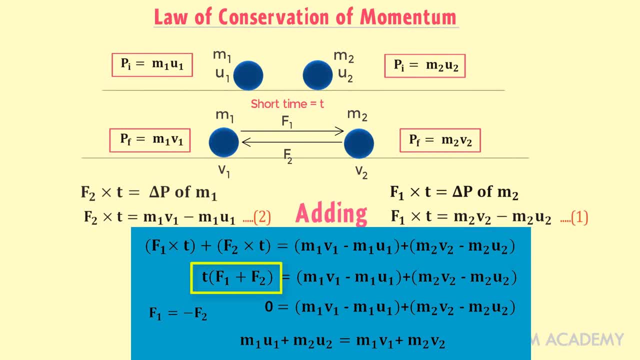 We are taking T as a common T: N2, F1, N2, F2 is equal to M1 V1 minus M1 U1 plus M2 V2 minus M2 U2.. F1 and F2 are equal in magnitude and opposite in direction, hence they are zero. 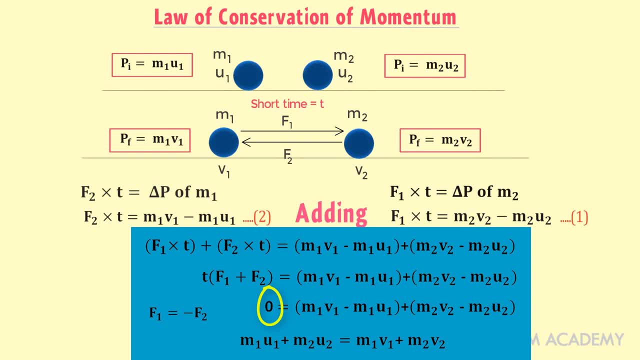 Thus left hand side becomes zero. Zero is equal to M1 V1 minus M1 U1, plus M2 V2 minus M2 U2.. Rearranging the equation and we get: M1 U1 minus M2 U2 is equal to M1 V2 minus M2 U2.. 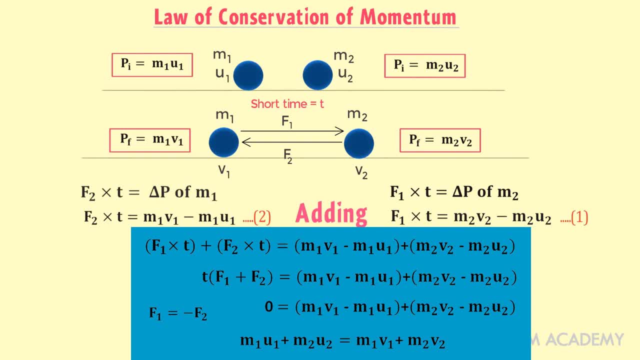 Rearranging the equation and we get: M1 U1 minus M2 U2 is equal to M1 V2 minus M2 U2.. We are taking T as a common F1, N2, T plus F2 N2. T is equal to M1 V1 plus M2 V2.. 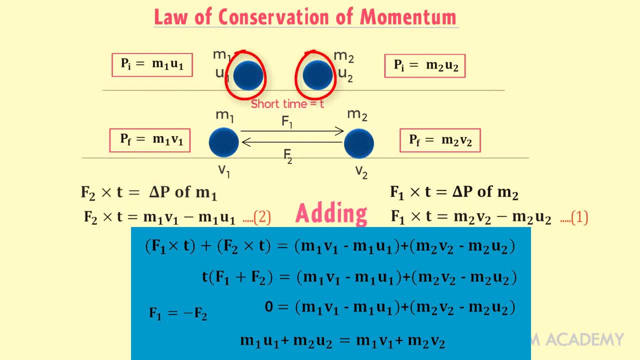 It means that the total momentum of the balls before collision are equal to the total momentum of the balls after collision. Thus, total momentum of the balls are constant in this isolated system. This law is known as a law of conservation of momentum. Thus, left hand side becomes zero. 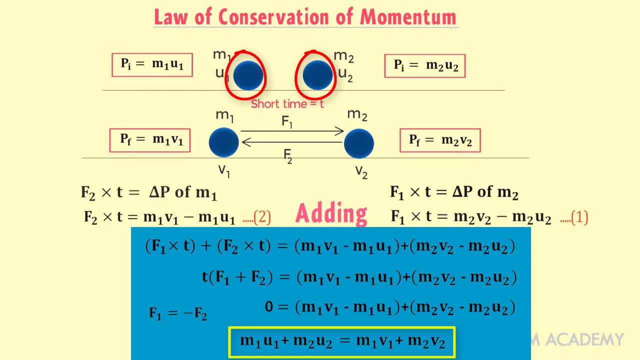